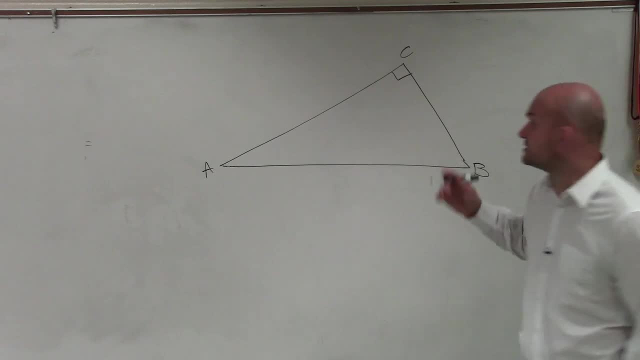 you label your triangles with large capital letters, and then the side lengths will be little A, little B and then little C. Okay, now what I'm going to show you how to do is how to create two other triangles that are similar to that. But to do that, I have to ask a very, very important question. And to do that I have to ask a very, very important person. Tyler, do you remember what the definition of altitude is for a triangle? Okay, for a triangle. 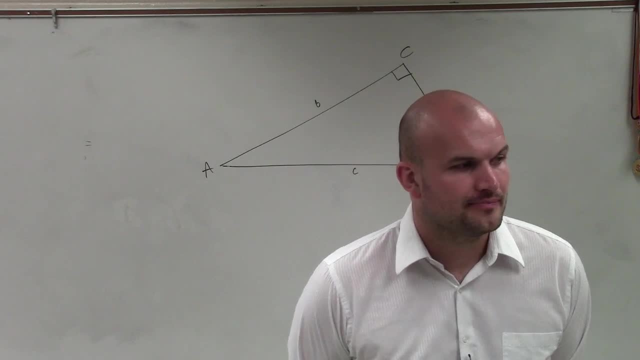 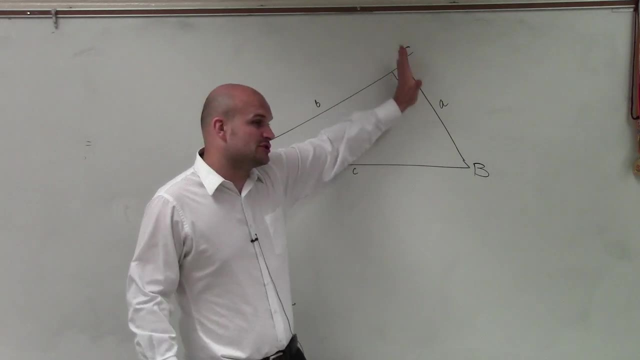 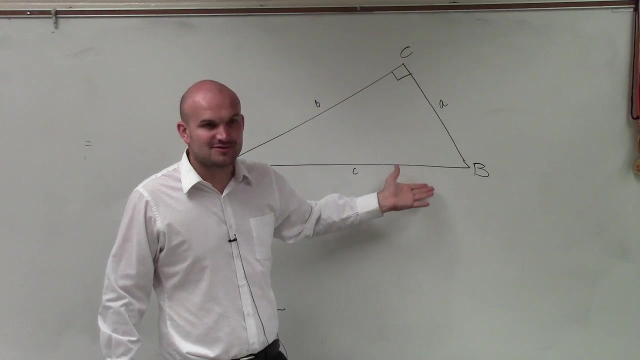 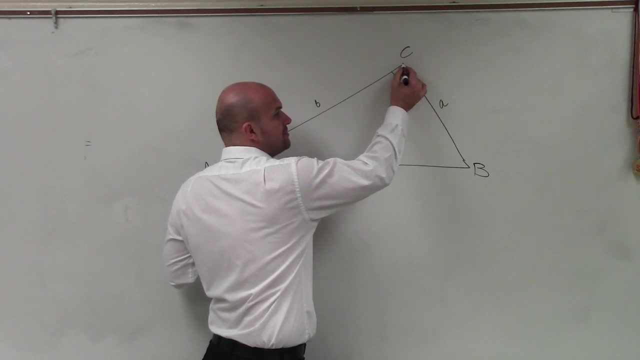 If you forget, Dustin, do you remember? From the midpoint straight down. It doesn't have to be from the midpoint, but what the altitude does tell us, though, is: yes, it is going to be a straight line. You're going from the top of the triangle to the base, And if you go from the top to the base, that distance would be what we call the altitude, which could also be thought of as the height. So if I go from the top straight down- and since I'm going straight down, that's going to create a perpendicular line. 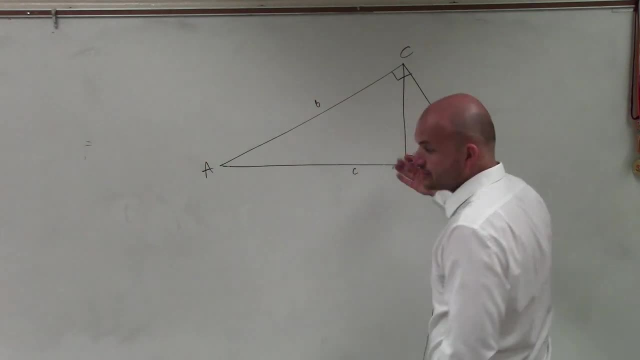 So if I go from the top straight down, and since I'm going straight down, that's going to create a perpendicular line with my base. So if one side's a right triangle, one side's a right angle, would that make sense that the other one's a right Right, Because the base has to be a line, correct? 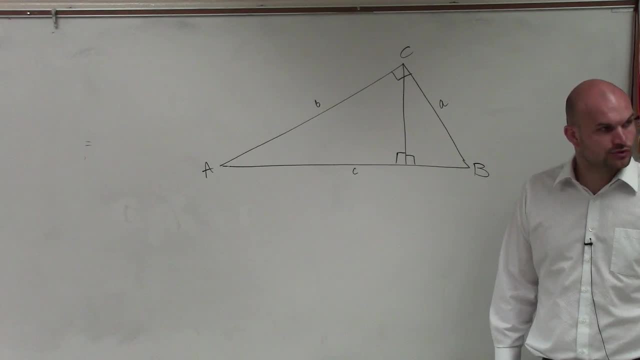 Alright, so does everybody see now that I've created two new triangles? Okay, So where that altitude came down, we're going to call D, and I'm going to call the altitude H, because that's going to represent the height. Alright, so that new point is D, and then actually this whole length, we're going to call C. 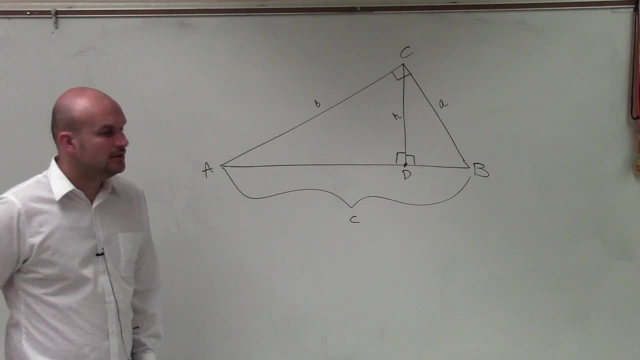 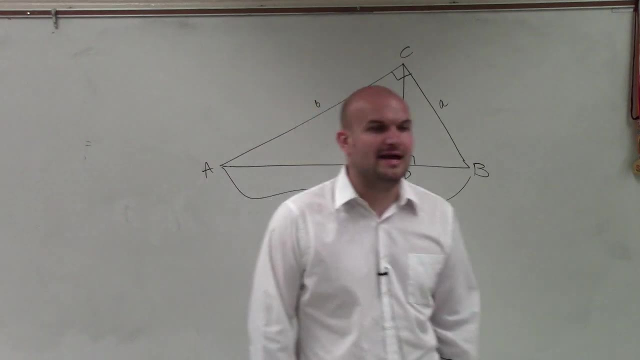 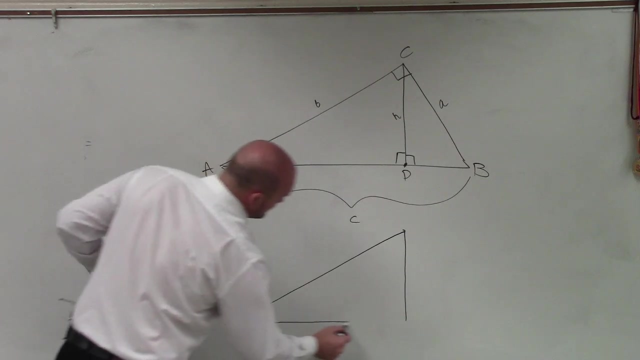 Okay, Everybody follow me so far, Okay. So what I want to do, though, is when we're looking at that big triangle, what we have just done is also created two other triangles that are very important. We create a triangle, and to show you how important they are, I'm going to redraw them separated. 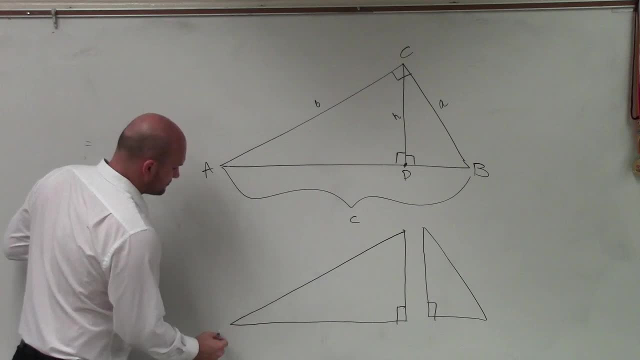 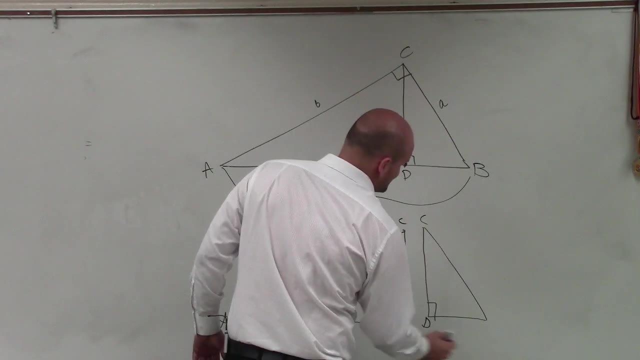 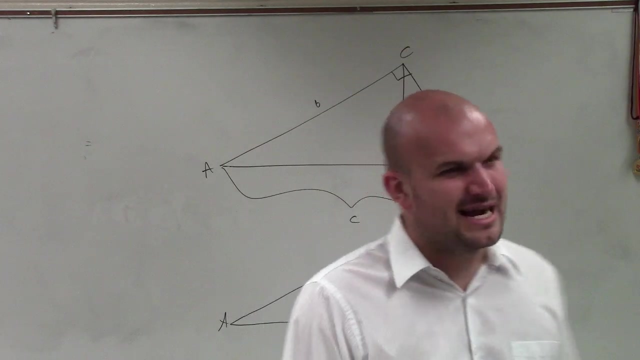 Now do these triangles look like they are the same shape, but not necessarily the same size? Yes, they both look like. they both look kind of. they have like the 30-60-90 triangle shape to them. right, They both look like they're similar triangles, but they're definitely not the same size. We can agree with that one. 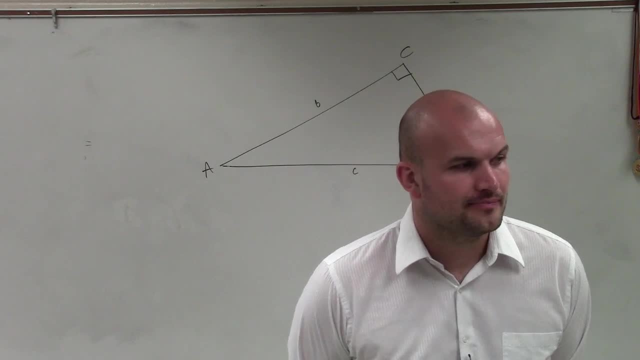 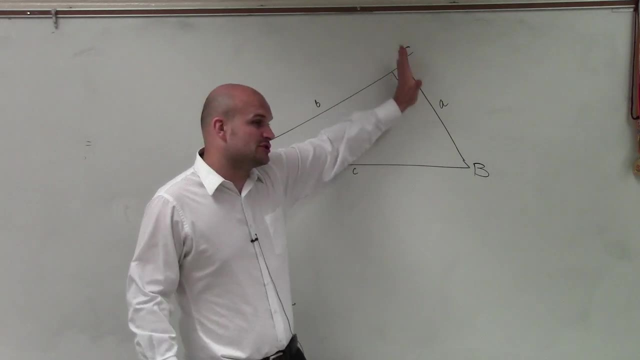 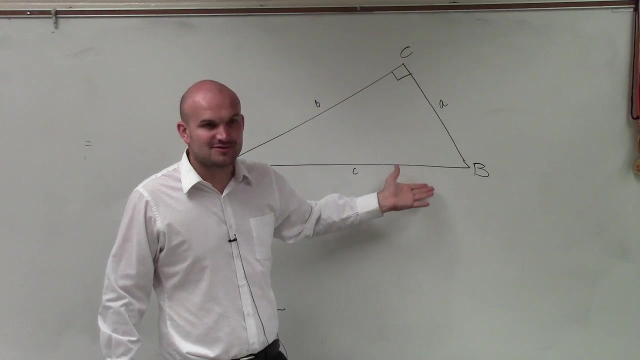 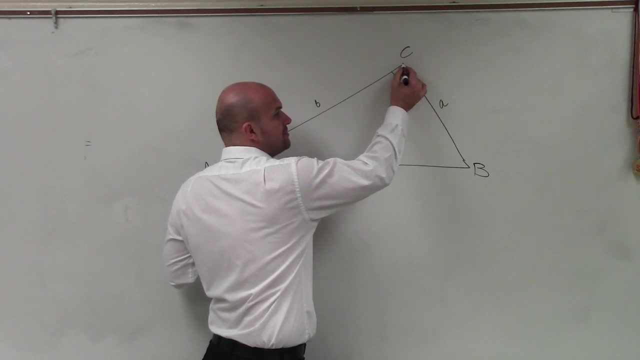 If you forget, Dustin, do you remember? From the midpoint straight down. It doesn't have to be from the midpoint, but what the altitude does tell us, though, is: yes, it is going to be a straight line. You're going from the top of the triangle to the base, And if you go from the top to the base, that distance would be what we call the altitude, which could also be thought of as the height. So if I go from the top straight down- and since I'm going straight down, that's going to create a perpendicular line. 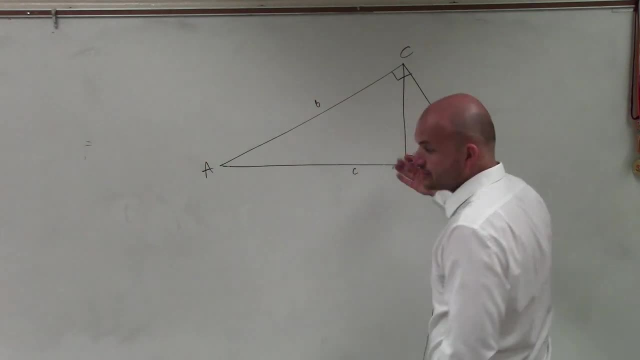 So if I go from the top straight down, and since I'm going straight down, that's going to create a perpendicular line with my base. So if one side's a right triangle, one side's a right angle, would that make sense that the other one's a right Right, Because the base has to be a line, correct? 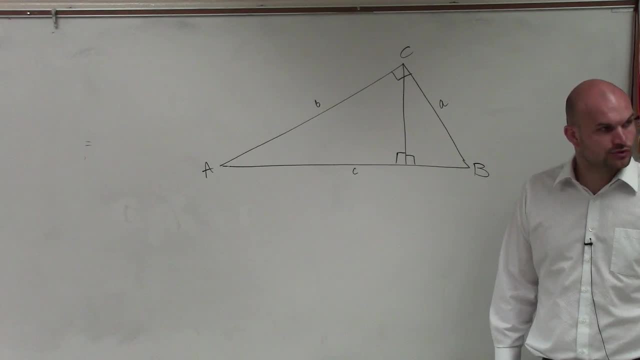 Alright, so does everybody see now that I've created two new triangles? Okay, So where that altitude came down, we're going to call D, and I'm going to call the altitude H, because that's going to represent the height. Alright, so that new point is D, and then actually this whole length, we're going to call C. 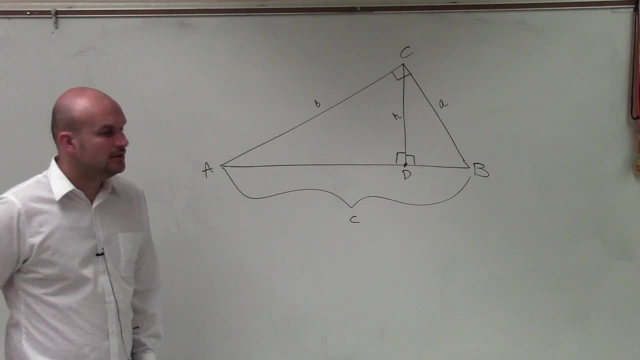 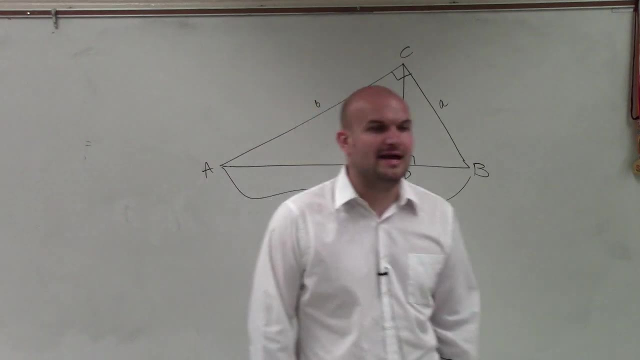 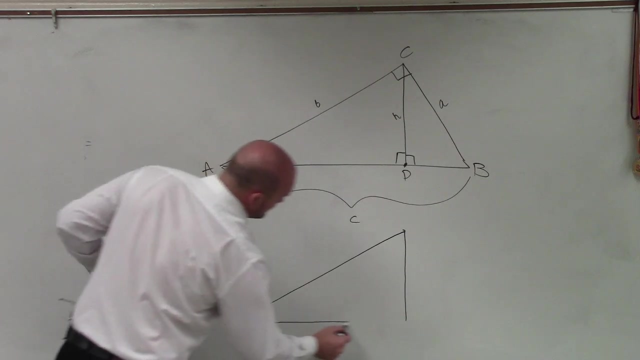 Okay, Everybody follow me so far, Okay. So what I want to do, though, is when we're looking at that big triangle, what we have just done is also created two other triangles that are very important. We create a triangle, and to show you how important they are, I'm going to redraw them separated. 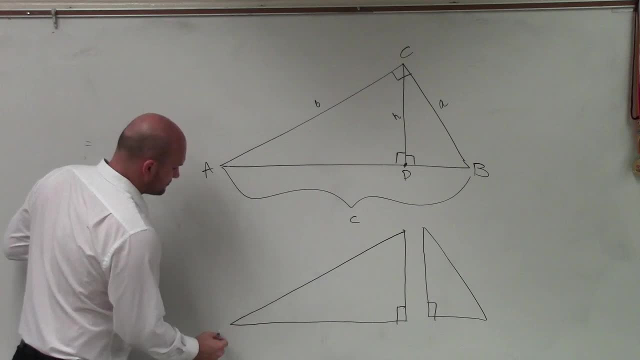 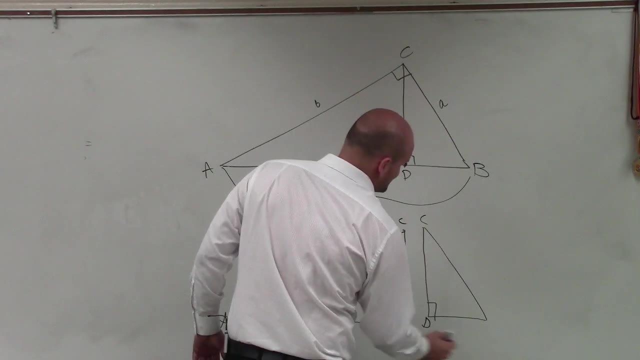 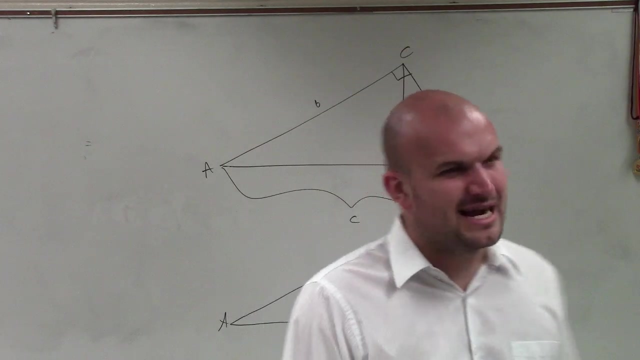 Now do these triangles look like they are the same shape, but not necessarily the same size? Yes, they both look like. they both look kind of. they have like the 30-60-90 triangle shape to them. right, They both look like they're similar triangles, but they're definitely not the same size. We can agree with that one. 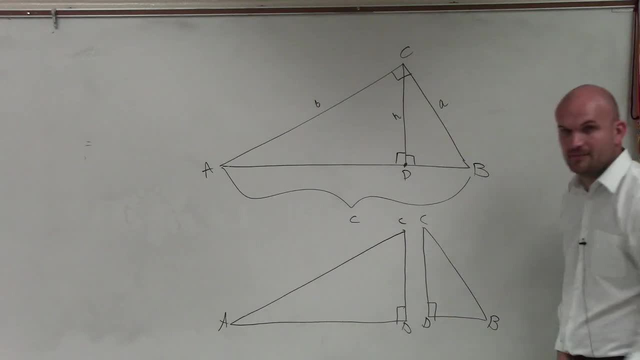 But does this triangle look like this one? but if I just tilted it over they'd kind of be definitely the same. Yeah, Yeah, but if I took this and flipped it like that, would it look? would it be more similar to that? 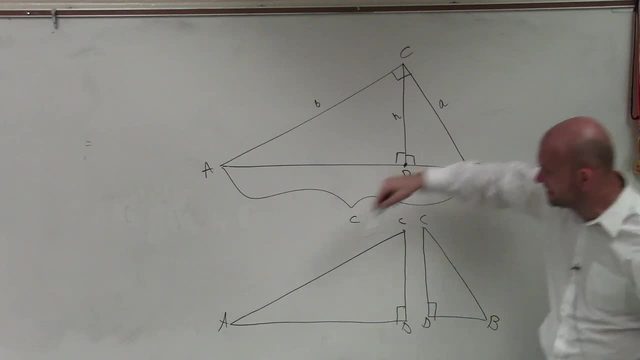 So, therefore, could you guys say: would it make sense, though, for me to say that C was the same angle as A? No, No, Corresponding, I'm sorry. not the same angle, but the corresponding angle. I can take this triangle and turn it to its side, and it's going to look just like that one, just obviously dilated. 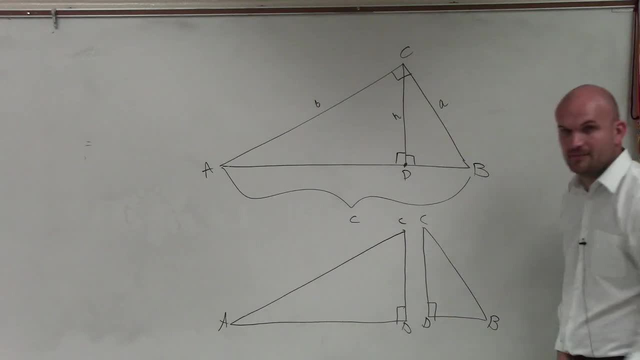 But does this triangle look like this one? but if I just tilted it over they'd kind of be definitely the same. Yeah, Yeah, but if I took this and flipped it like that, would it look? would it be more similar to that? 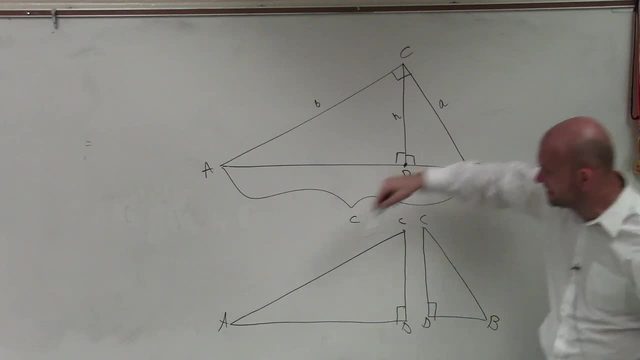 So, therefore, could you guys say: would it make sense, though, for me to say that C was the same angle as A? No, No, Corresponding, I'm sorry. not the same angle, but the corresponding angle. I can take this triangle and turn it to its side, and it's going to look just like that one, just obviously dilated. 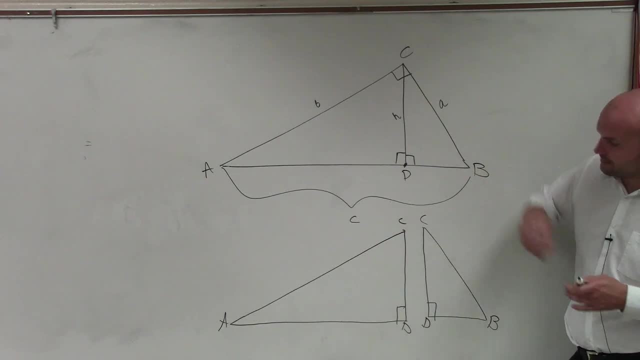 Yeah, Yes, Okay. Now can we wait two seconds for that? please Just wait. Just wait for two seconds, right, Okay? So now the next thing I want to look at is: let's look at this big triangle, the big right triangle. 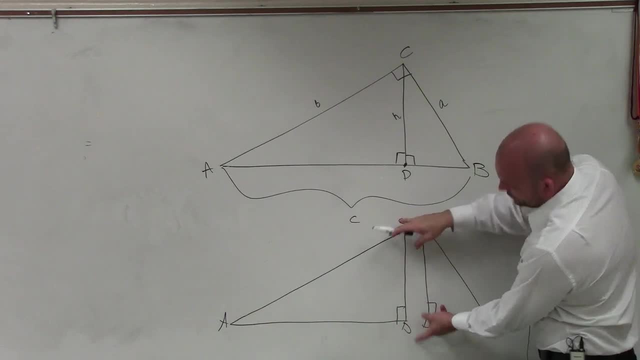 Is that kind of like this one, but like if I took this triangle and flipped it over, then that would look kind of similar to that one. If I took this one and wrote and reflected it over the hypotenuse, it would kind of be the similar figure as that. 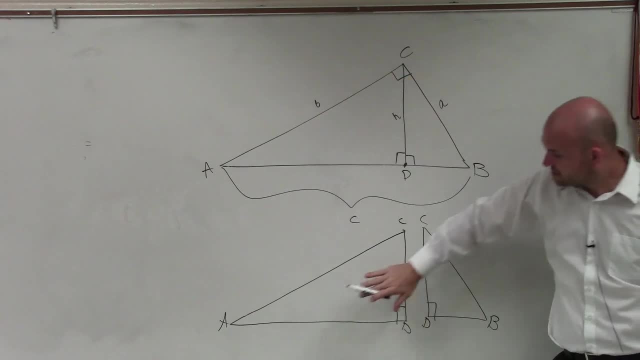 Obviously, it's not the same size, but it's the same shape. Yeah, Take this and flip it over And it would look something similar to that. What I'm trying to show you, guys is: these are all right triangles, If we can maybe forget about this for a second. 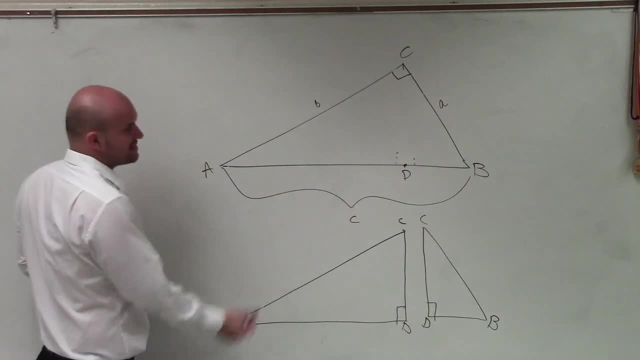 I got these two triangles from up here. What I want you guys to see is all three of these right triangles are all similar. Obviously, that's the largest, That's the next largest And then that's the smallest, But what's so important is these are all similar. 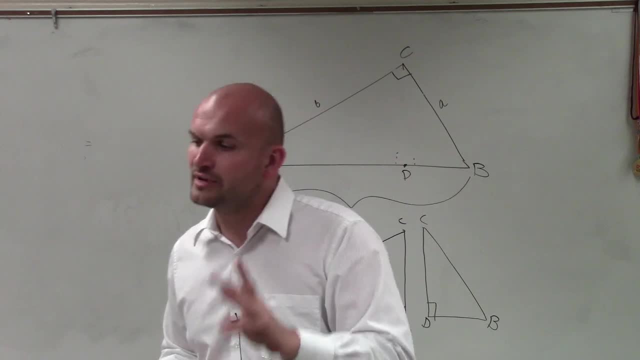 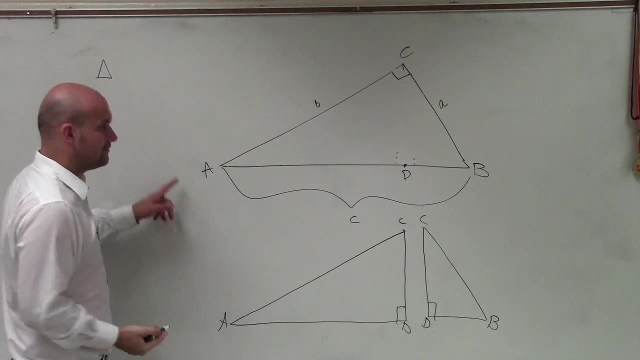 So when you create your altitude, what you do is you create three similar triangles So we can write a similarity statement. So the first one, I'm going to start with A C B, So triangle A C B. Now, as I mentioned, this triangle is the same as this one kind of like rotated out. 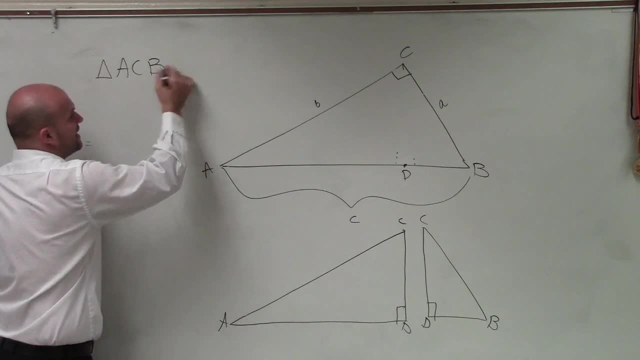 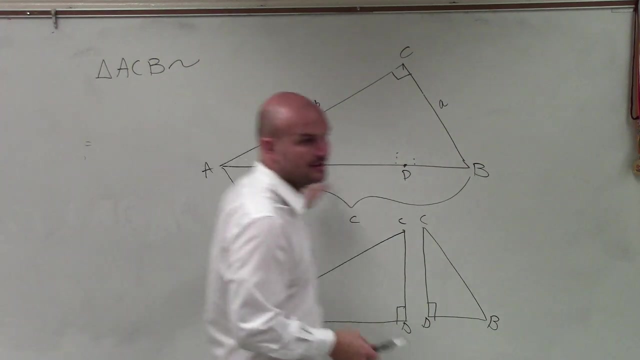 So if I'm going to say triangle A, C, B is similar, what is the corresponding angle from this triangle to this triangle? What is the corresponding angle from this triangle to this triangle E? What is the corresponding angle for A? From this triangle to this triangle? what's the corresponding angle for A? 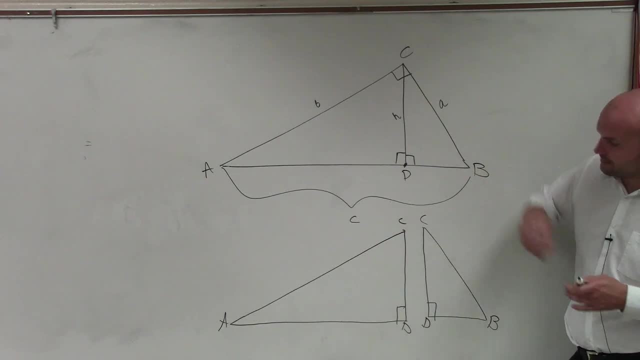 Yeah, Yes, Okay. Now can we wait two seconds for that? please Just wait. Just wait for two seconds, right, Okay? So now the next thing I want to look at is: let's look at this big triangle, the big right triangle. 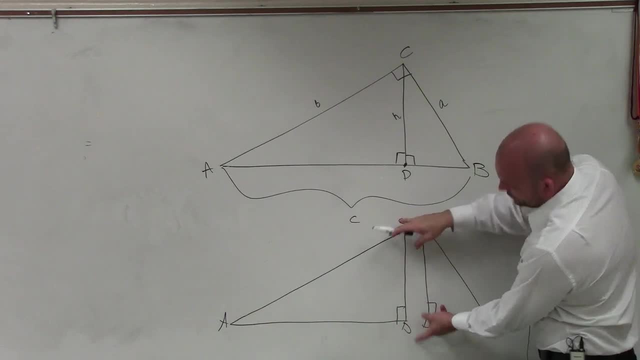 Is that kind of like this one, but like if I took this triangle and flipped it over, then that would look kind of similar to that one. If I took this one and wrote and reflected it over the hypotenuse, it would kind of be the similar figure as that. 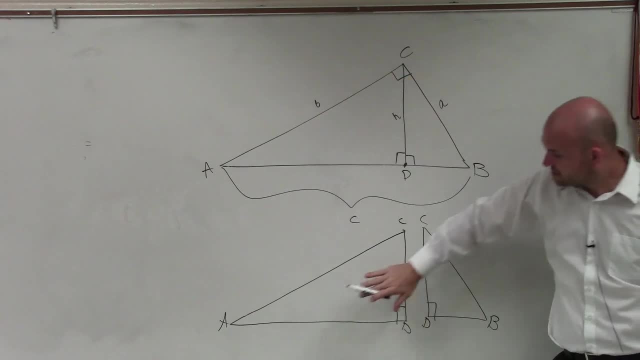 Obviously, it's not the same size, but it's the same shape. Yeah, Take this and flip it over And it would look something similar to that. What I'm trying to show you, guys is: these are all right triangles, If we can maybe forget about this for a second. 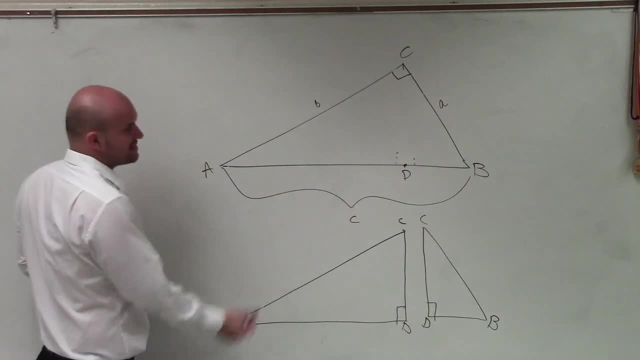 I got these two triangles from up here. What I want you guys to see is all three of these right triangles are all similar. Obviously, that's the largest, That's the next largest And then that's the smallest, But what's so important is these are all similar. 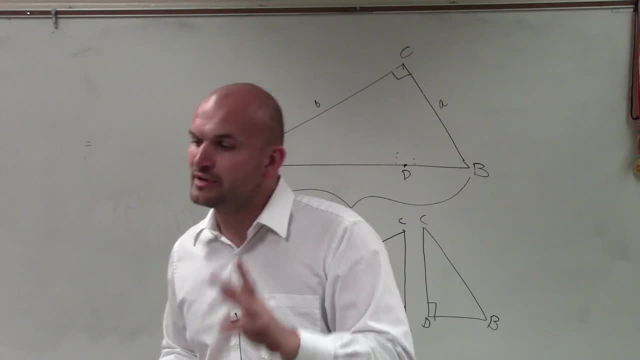 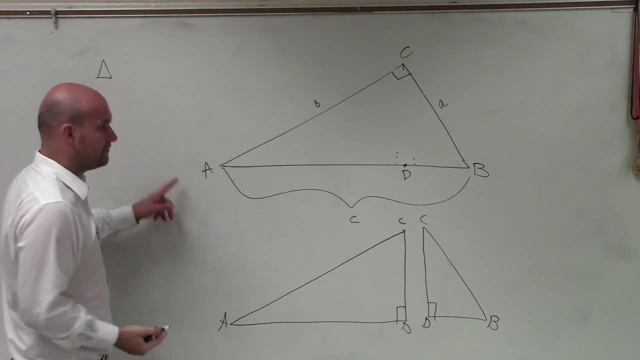 So when you create your altitude, what you do is you create three similar triangles So we can write a similarity statement. So the first one. I'm going to start with ACB, So triangle, ACB. Now, as I mentioned, this triangle is the same as this, one kind of like rotated out. 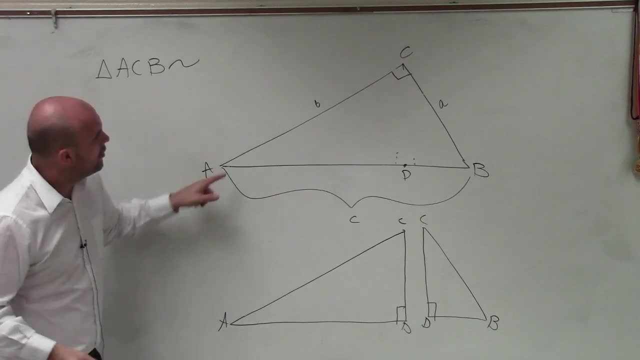 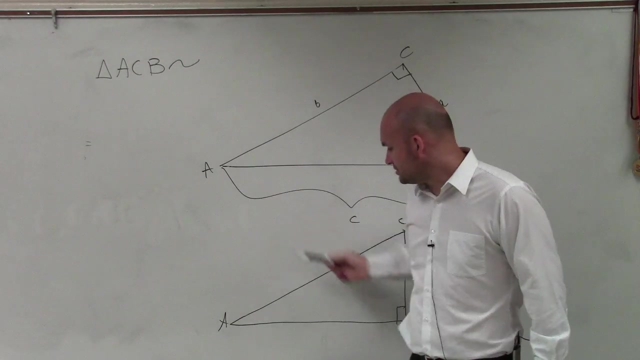 So if I'm going to say triangle ACB is similar, what is the corresponding angle from this triangle to this triangle B? What is this? This is the corresponding angle for A. From this triangle to this triangle. what's the corresponding angle for A? 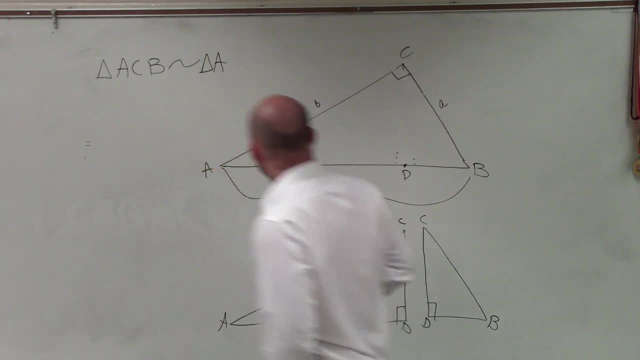 It's A. What's the corresponding angle for my right angle C for this triangle D, Because D is the right angle, right, And then obviously you can see B is at the end of the short leg here. What angle is at the end of the short leg for this one? 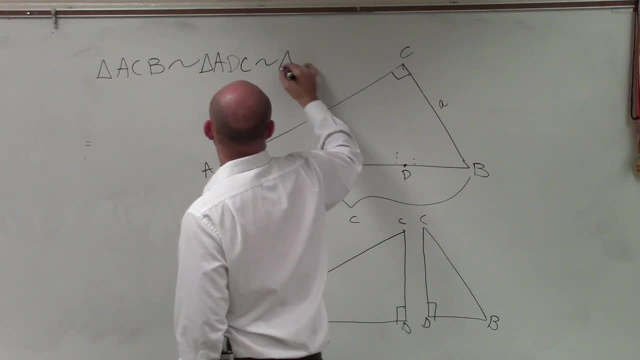 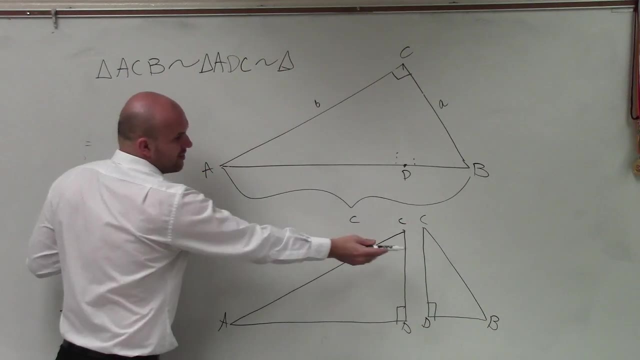 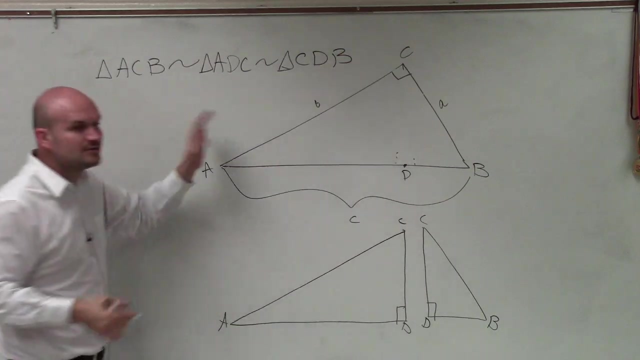 C, And that's also similar. So now remember we already said, this triangle is like this one, tipped over. So therefore, A corresponds to what angle over here, C, D, Because that's the right angle, And then B. So these three triangles are all similar to each other.